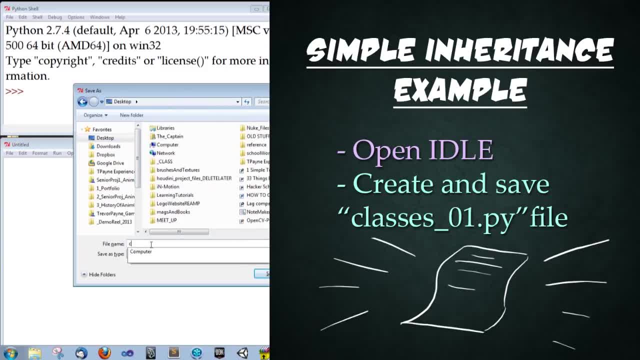 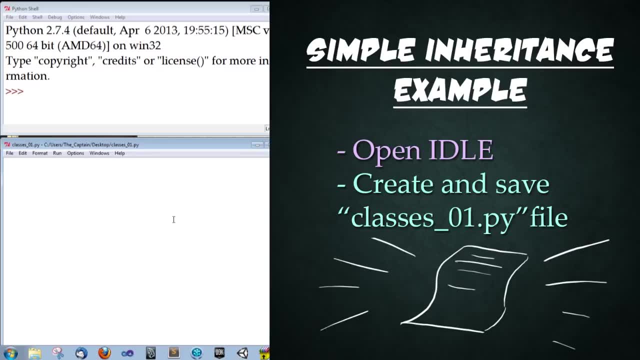 ahead and create a new file. Save this on my desktop as classes underscore zero one: dot py. Make sure you save with that dot py extension so it saves as a Python file. So first we're gonna create a base class and then we're gonna create an. 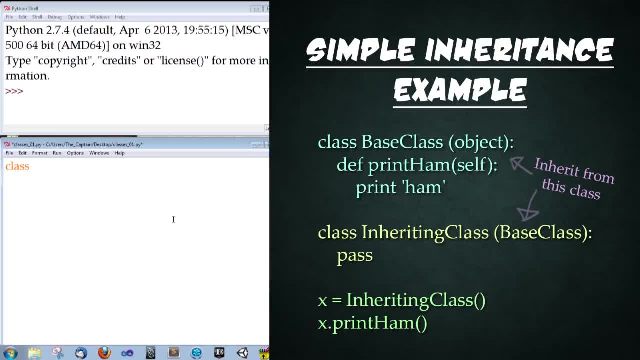 inheriting class. So let's type class, space, capital B for base and capital C for class, and then open parentheses, object, close parentheses and end with a colon. So what this is doing is this is creating a class called base class that is inheriting from object. An object is a base class stored somewhere within. 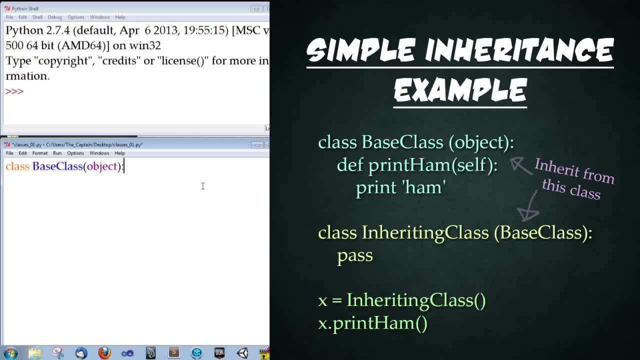 Python that allows inheritance to actually happen. All right, so next press ENTER and type DEF space, print and then uppercase ham. open parentheses, self. close parentheses. colon. enter whoops, misspelled def there. and then we're gonna type print and of course ham, because we love ham. 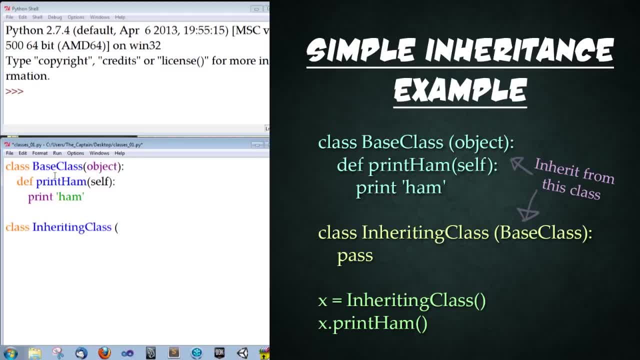 So next we're gonna type class: inheriting class- open parentheses- base class- close parentheses, colon enter, pass, enter, enter. So what this is doing is it's creating an inheriting class that will inherit from the base class. 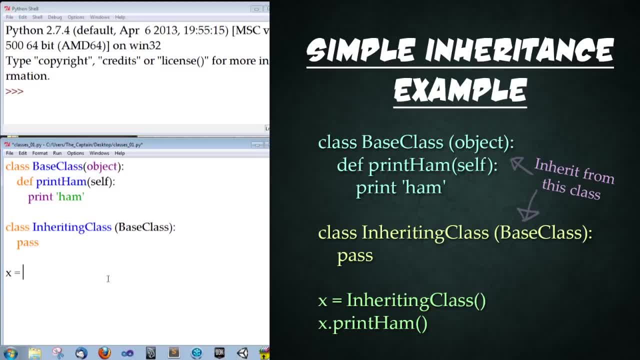 Okay, so next we're gonna type in at the bottom unindented. we're gonna type x, equals, and then create an instance of the inheriting class Open- close parentheses. enter x and then we're gonna access the function created within the base class. 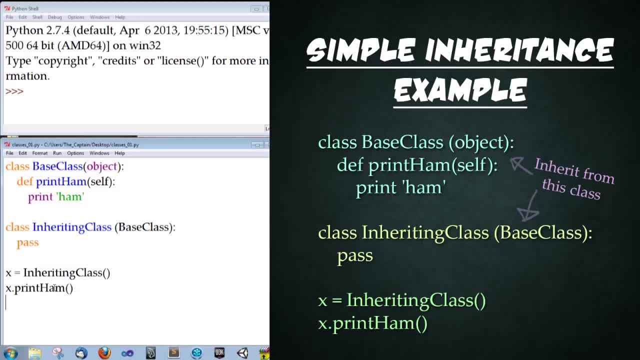 that's just called print ham: Open, close parentheses, enter save and then press F5 to run it. Perfect, so our program worked beautifully. We created an instance of this inheriting class and then called the function that was created within the base class. 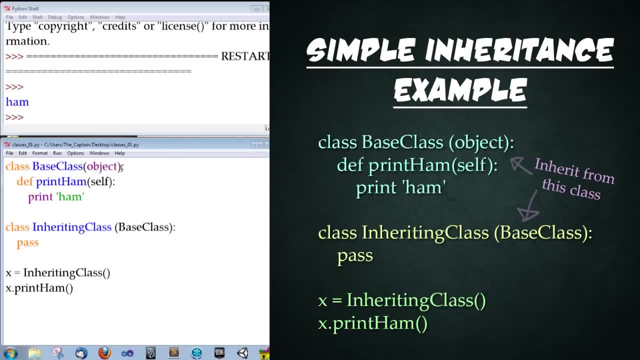 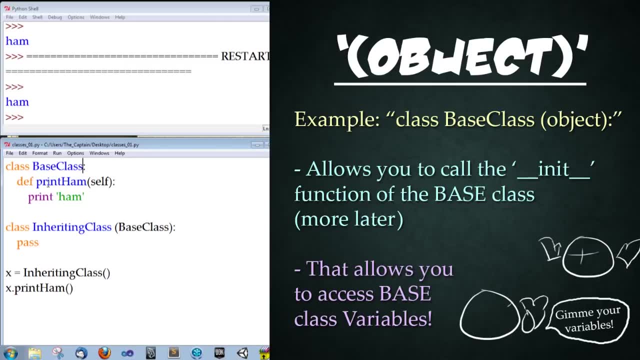 Now what happens if we didn't have this object here? I'm gonna go ahead and delete it, and you don't have to, but watch what happens. Notice that the program actually compiled correctly, and the reason being is it's inheriting the functions. 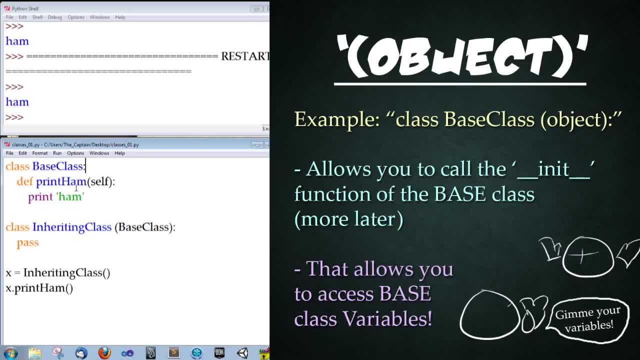 but we're not actually accessing any variables or attributes within this class, So that's why it compiled correctly. As a good practice, I would recommend always leaving in this base object in here, because when you try to call its init function from this inheriting class, it will not compile. 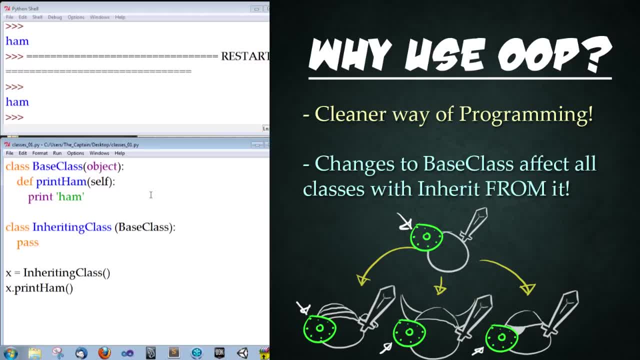 All right. so why use object oriented programming? Well, it's a much cleaner way of programming. For instance, if we wanted to make any changes to the base class, it would affect all the inheriting classes. So, for instance, if we were to create a character class, 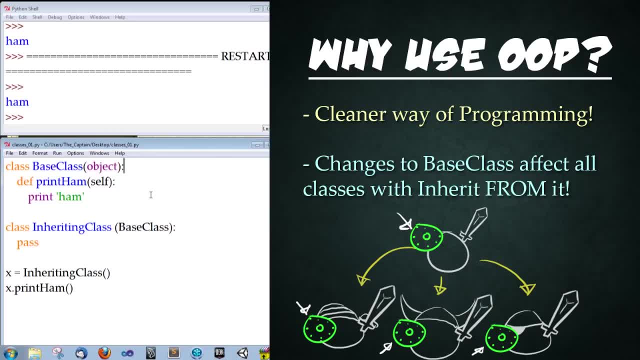 a base character class, which we will hear in a minute. if we wanted to change the health of all the characters across the board at once, or if we wanted to add new ability to all characters at once, we could do that with inheritance. 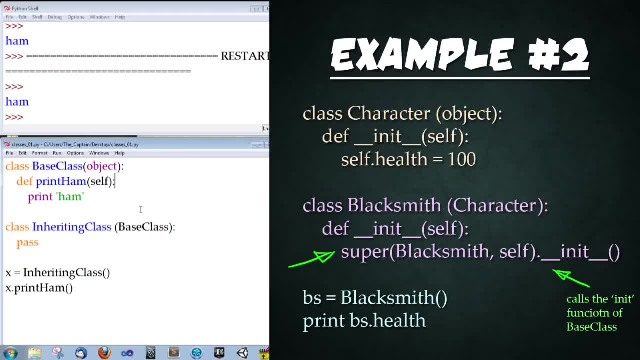 So let's go ahead and try another example. I'm just gonna go ahead and select all and delete it To create a fresh new file. We're gonna begin by creating a base character class and then we're gonna create a more specific character class. 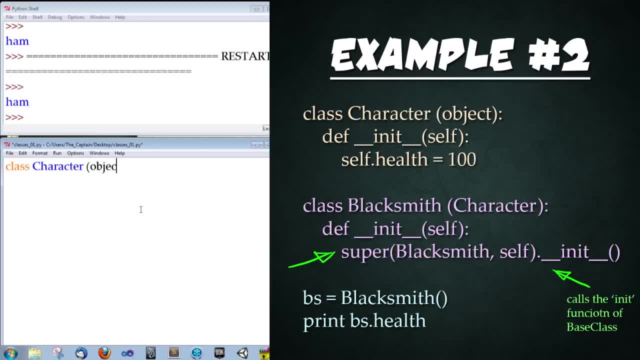 So first we're gonna type in class character- open parentheses, object. close parentheses. colon enter, def, underscore, init to call the constructor self colon enter. and then we're gonna create an attribute called health. Selfhealth is equal to 100, perfect. 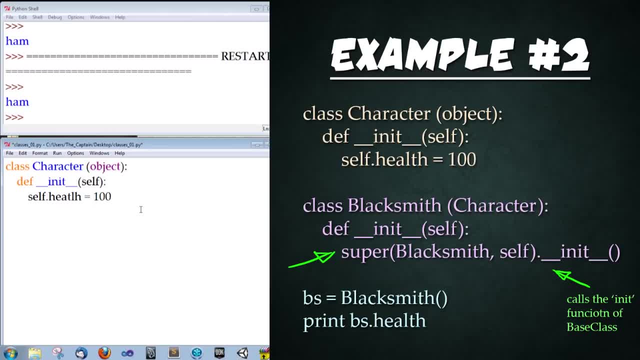 And that's it. we've created a simple base class and now we're gonna go ahead and create the inheriting class. So class blackhealth, Blacksmith- open parentheses- character. close parentheses- colon. and this is so that we inherit. 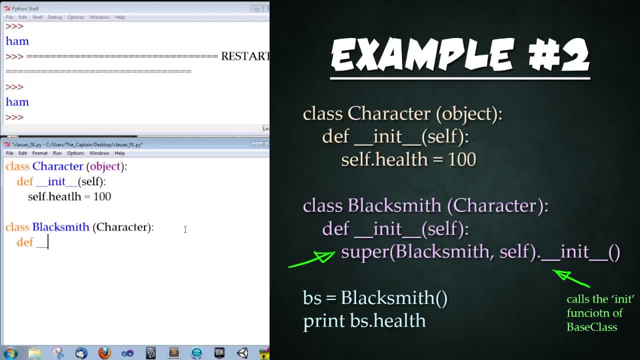 from that base class up above: enter. and then we're gonna go ahead and create a constructor for this one as well, with double underscore: init, double underscore. we're gonna type self again, colon enter. next we're gonna be calling an odd function. 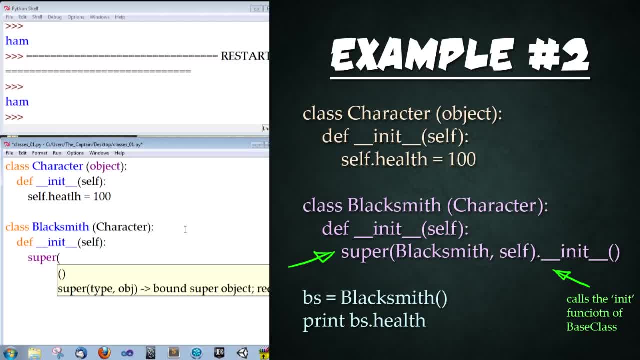 we haven't seen before. We're gonna type in super open parentheses and then type in the class name that we are currently in. So we're gonna type in blacksmith, comma space self close parentheses and then we're gonna type in: 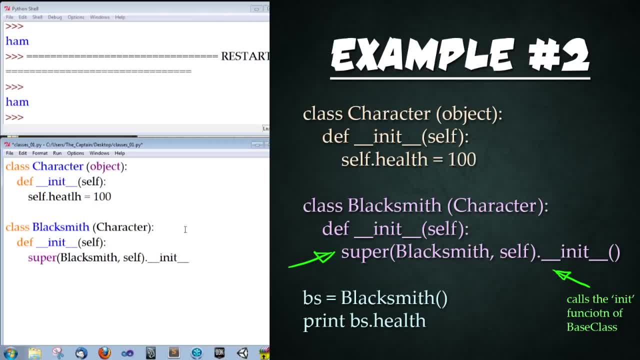 dot, underscore, underscore, init, underscore, underscore- to access the constructor and then end with open, close parentheses. So what this is gonna do is it's gonna call the init function from the base class that we inherited from. So go ahead and unindent back down. enter, enter. 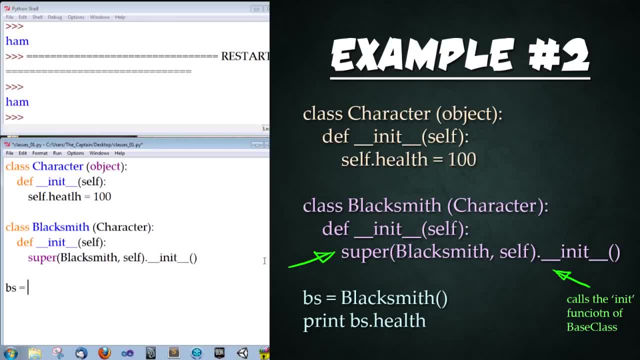 and then we're gonna go ahead and create an instance of that class by typing bs equals blacksmith, open, close parentheses, enter and then print bshealth- Save, run it. so we ran into a compiler error and it's saying that: ah, I don't know, I don't know. 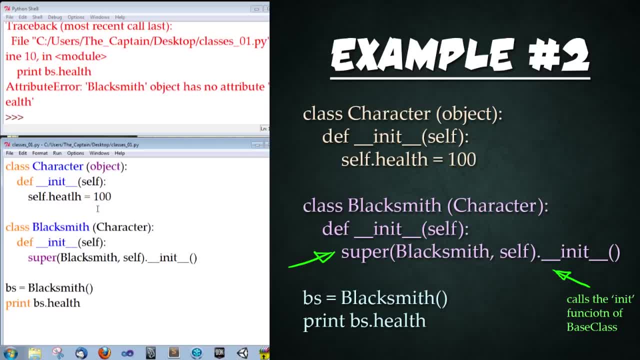 it has no attribute health. That's because I did a misspelling up here, So I'm gonna go ahead and fix that. Save run perfect. So this worked out perfectly. Now, what happens if we were to delete this in this object? that's inheriting. 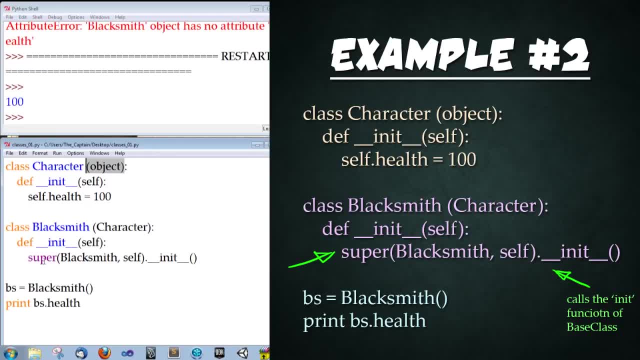 Now we would not be able to use this function, super, to call the init function from the base class. So let's go ahead and delete it, run it, and now we get that error I was expecting, in which it's saying that there is no base class objects. 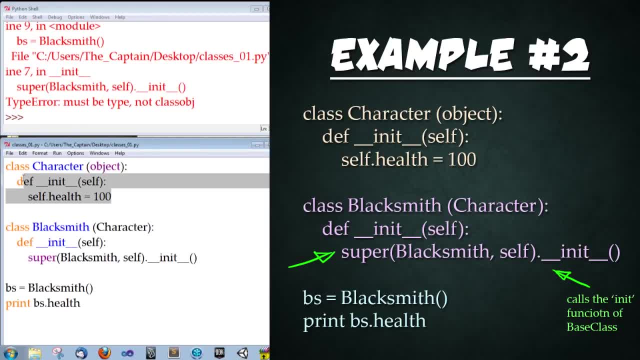 As a note, you don't have that in there. if you're gonna be calling the init function from the base character. Can't tell you how many times I've run into errors because of that. All right, so this can get kind of messy. 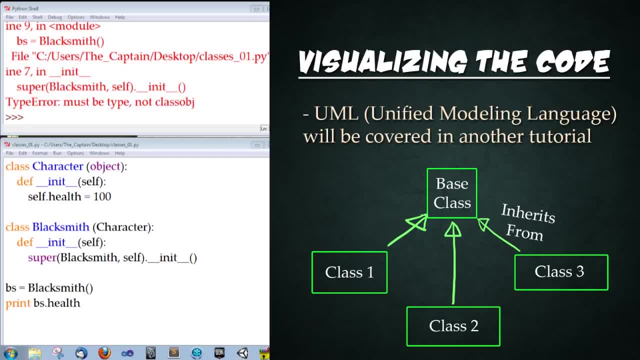 So what helps is usually to draw out a diagram to visualize what's going on with the inheritance. So the best way to visualize is using UML, and I'll get into that in another lesson, but here's basically what you need to know. 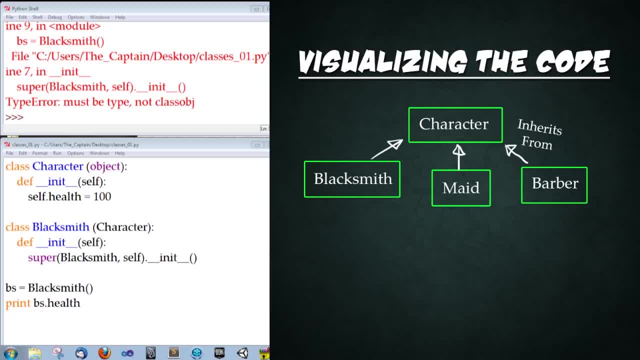 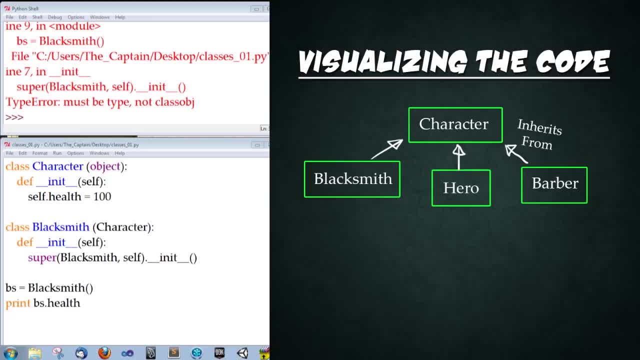 Let's say we wanted to add a hero class as well. That would also inherit from the base character class. but let's say there's more than one type of hero. Let's say we have an archer, a sorceress and an ugly man. 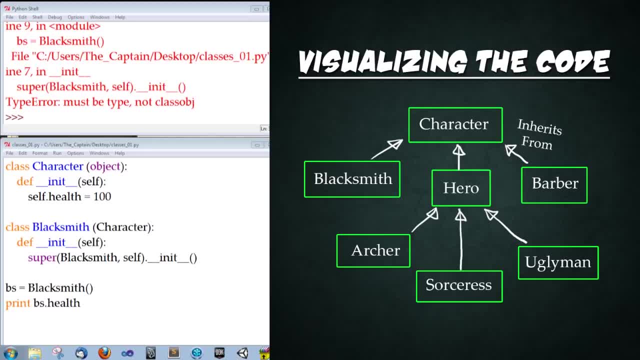 An ugly man isn't the character you want to be, but they would all inherit from the hero class. So you can see that we can hierarchically build downward and the final challenges will have more cases just like this. So let's further expand on our past example. 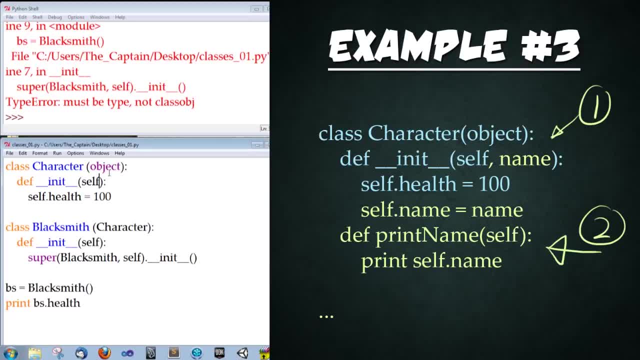 to include inherited functions. So in the character class, which is the base class, I'm gonna go ahead and add in a parameter called name into the constructor or the init function. Next I'm going to secure it to the instance of the class. 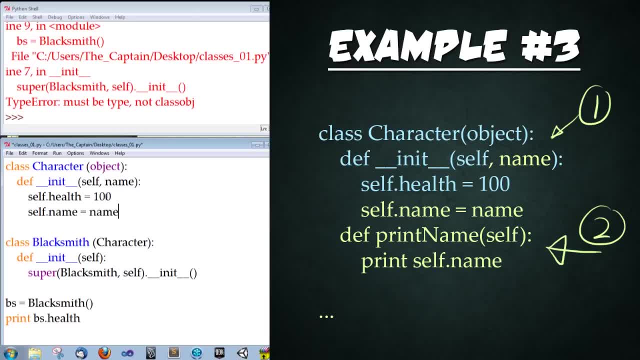 by using selfname is equal to name, and this is just creating another variable and attaching the passed in variable to it. Finally, I'm going to create another function that's called def, print, name, self. in the arguments colon enter print and then selfname. 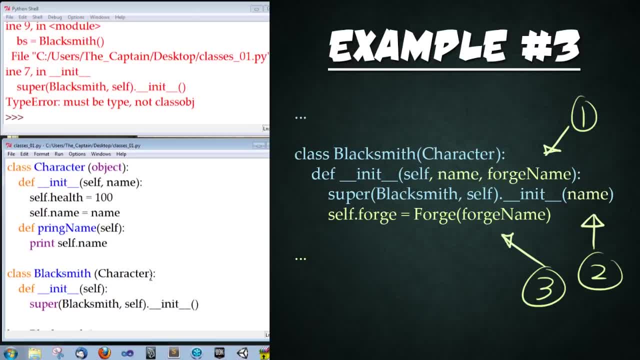 This is just a simple function that's gonna print out its own name. Cool. so in the blacksmith class I'm gonna make the following changes In the arguments of the constructor: I'm gonna add in name comma, forge name. 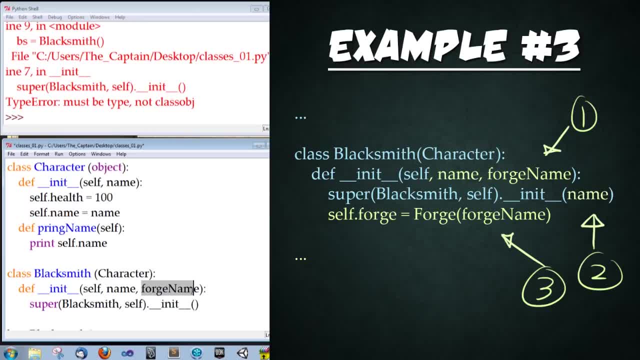 The name is gonna be the name of the character and the forge name is gonna be the name of the forge. that's gonna be stored within the character. All right, and we're gonna go ahead and pass down that name. that's passed in the parameters. 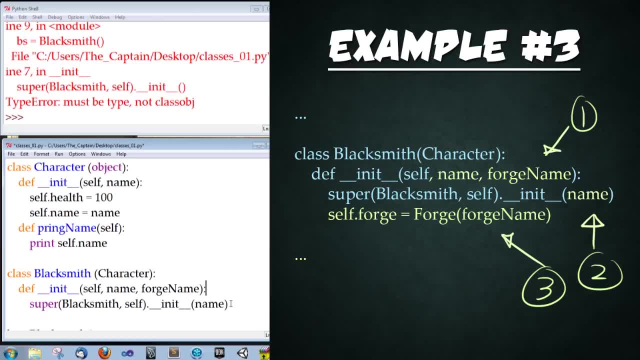 of the init function into the base class init. The reason being is we're calling the init function of the base class, so we wanna pass in the parameters that are associated with it. Finally, we're gonna type in: selfforge is equal to. 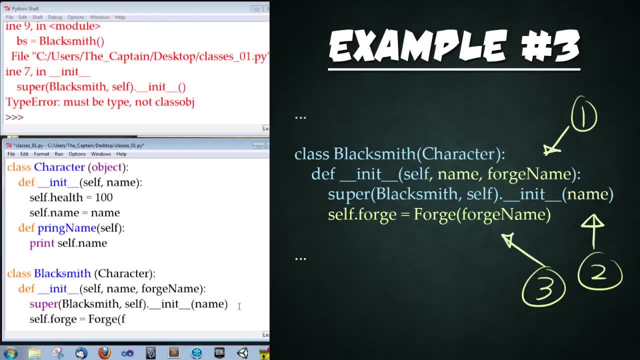 and then capital F-O-R-G-E and then type in lowercase F-O-R-G-E. This is gonna be calling an uppercase N for name and this is a class we're gonna create here in a minute. Okay, so scrolling down. 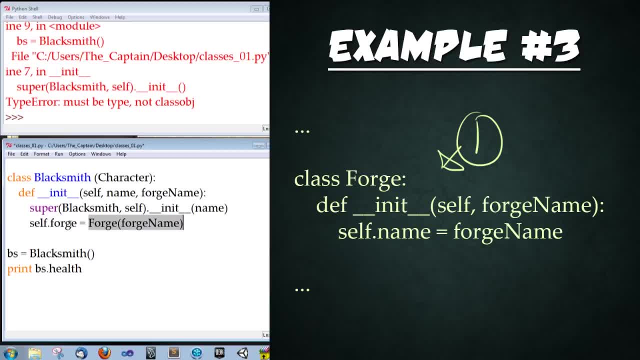 In this instance, we're gonna be storing an instance of the forge class within the blacksmith himself, So let's go ahead and create that forge class real quick. Gonna go enter. enter. enter. Type: class: forge- open parentheses. colon enter. 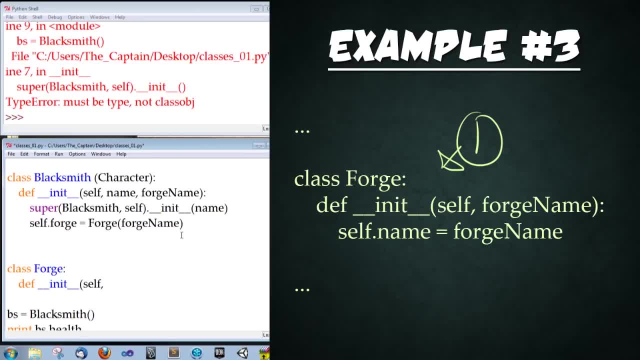 def. underscore, underscore, init. underscore, underscore, self comma, forge name, close parentheses, colon enter and then selfname is equal to forge name, And this is merely so we can stick that name and attach it to this instance of the class. 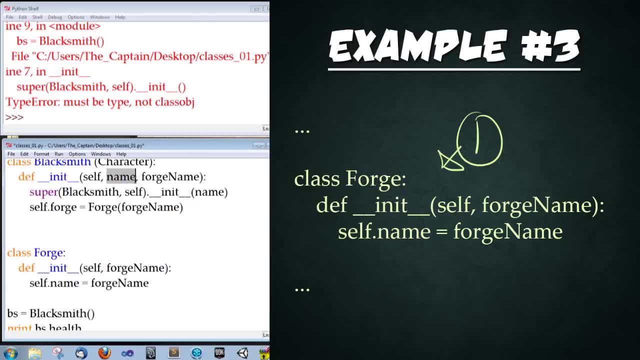 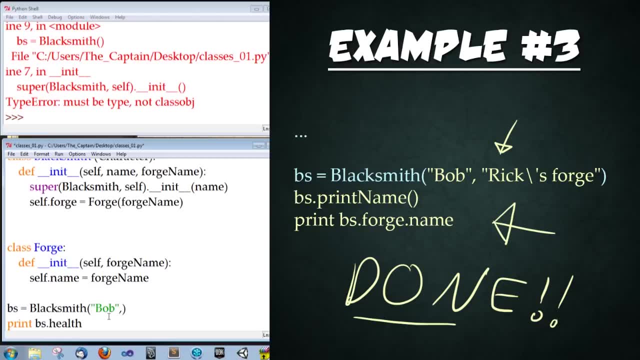 Perfect. So now that we've changed the constructor of the blacksmith class, we need to include parameters within the call of the function. So for the first parameter or name, I'm gonna create Bob comma and then we're gonna enter in the forge's name. 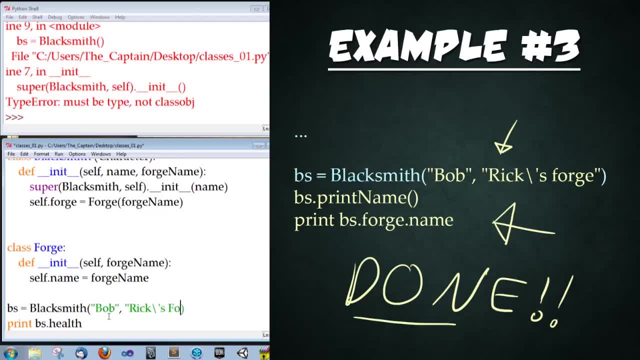 and that's gonna be Rick's backslash for the parentheses forge. You can name it whatever you'd like. The reason is: Bob killed Rick and took over his forge, so that's why it's called Rick's forge. Finally, we're gonna go ahead and call. 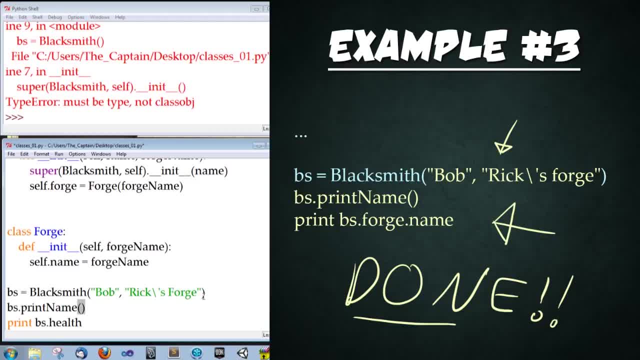 bsprint name. open close parentheses to call that function we created in the base class bsprint name. And, lastly, I'm gonna print the forge name so we can make sure that it's working. so, forgename. so that way we're gonna be accessing. 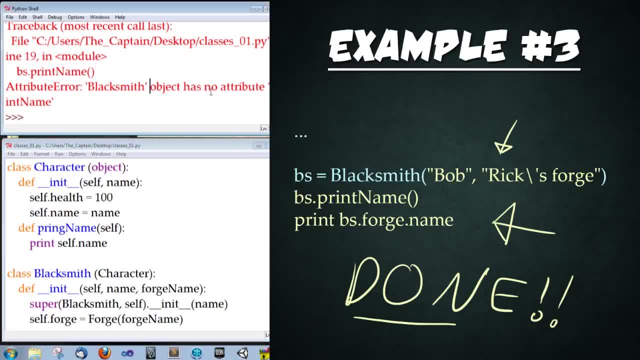 the forge and then the name. So I ran into a small error in which it said there's no attribute print name and that's because I did a slight spelling error right there. I'm gonna go ahead and fix that. rerun it perfect. 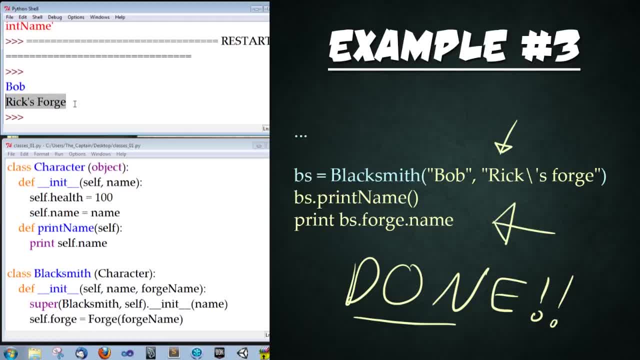 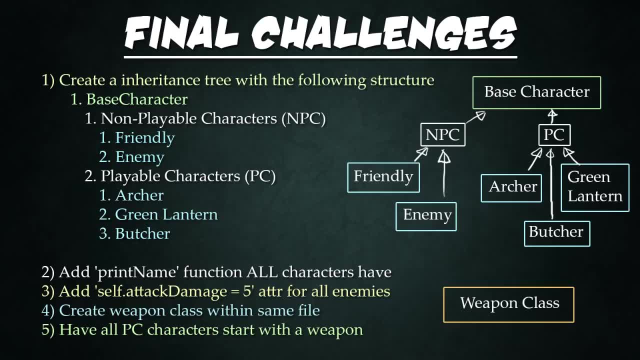 So we can see Bob is printed out, the character's name and also Rick's forge is printed out. Perfect, Excellent. so that's all for part one of the object-oriented programming. Thank you so much for watching and great job keeping up.